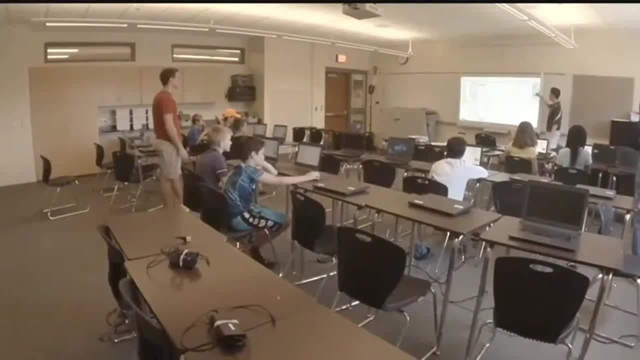 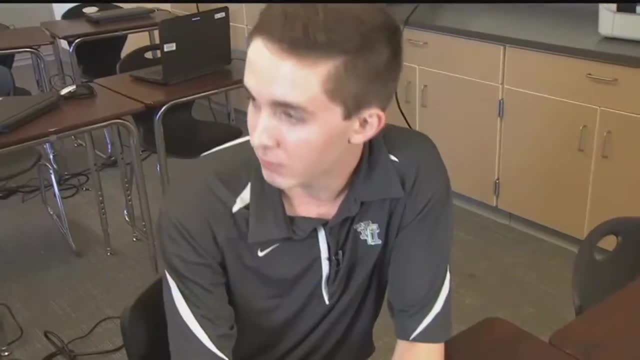 The first and foremost reason for why we want to target these younger generations is because they have the creative solutions and they have the vision. So what we want to do is combine that with the practical knowledge on how to make it happen. It seems kind of hard. 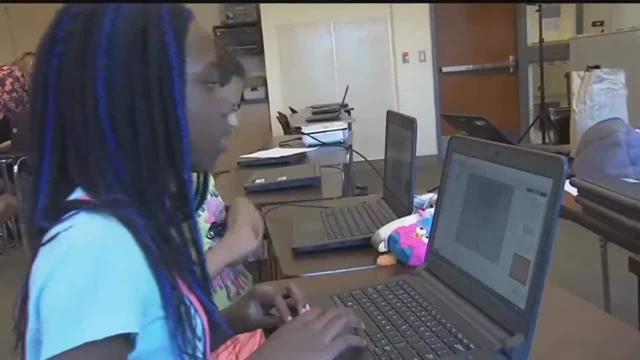 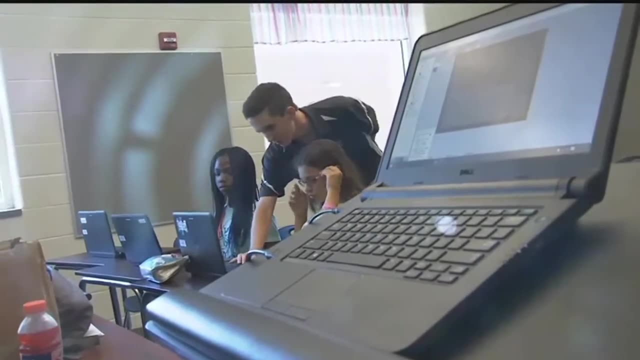 Well it is, but we have help from the counselors. There's definitely a need for females. Here at YouthSec we have a class targeted towards females, our Gaming Gals class, But We definitely want to make females to feel like they have a place in coding and in computer programming. 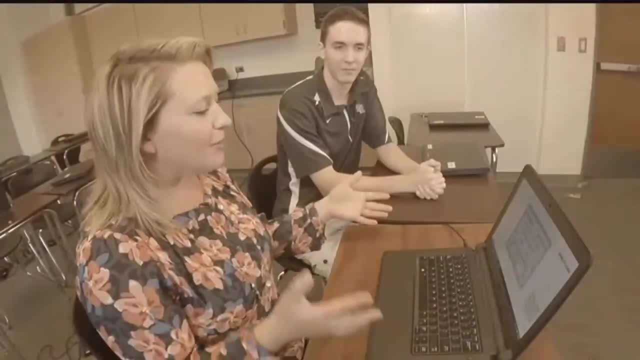 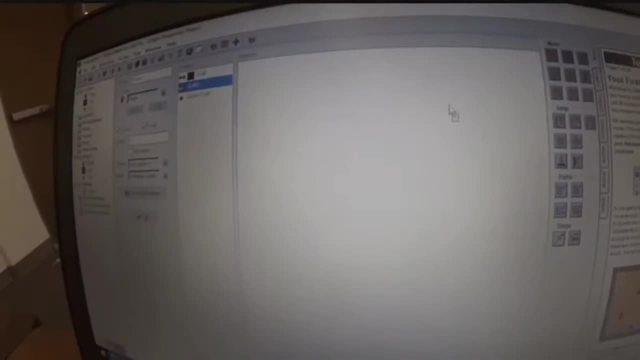 because definitely everyone's needed to make it work together. You have a game set up here and you're going to kind of teach me how to code a little bit. We're going to go to this keyboard event here, Okay, And then we're going to go to left. 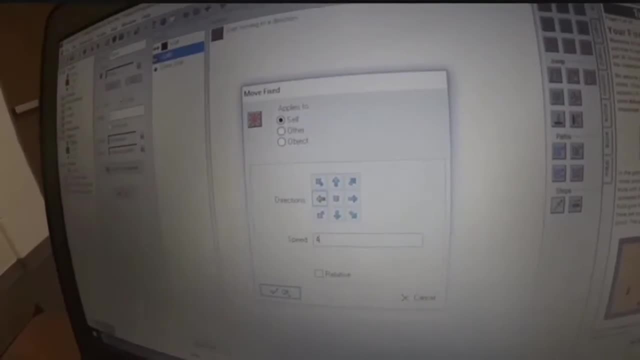 Uh-huh. And basically now we're saying, whenever you hit the left arrow key, you're going to perform whatever is in your actions. Cool, Okay. so now that we have the up down right left, can we play the game? 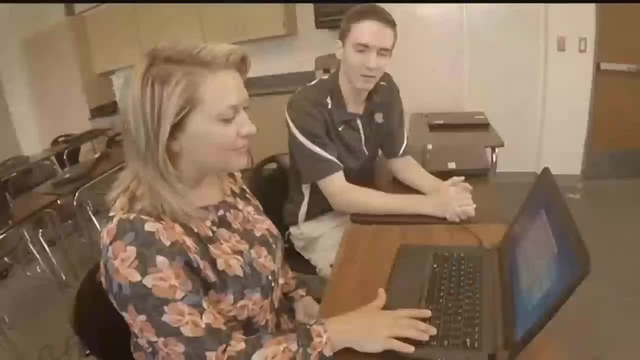 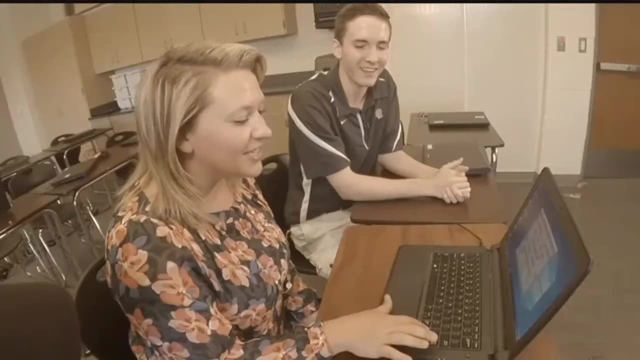 Well, let's test it out. Okay, so I'm going to try. You're going to go up With the arrow key? Oh, That's okay. Yeah, don't press space. Press the arrow key, Oh no. 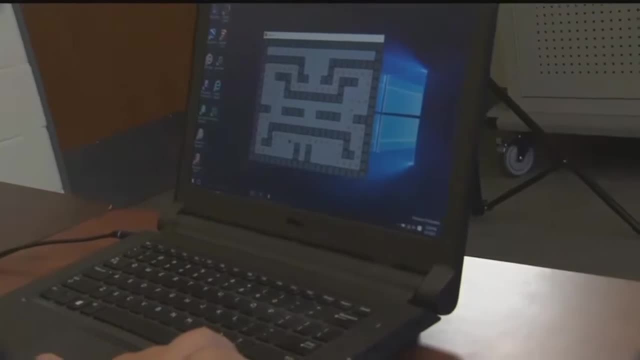 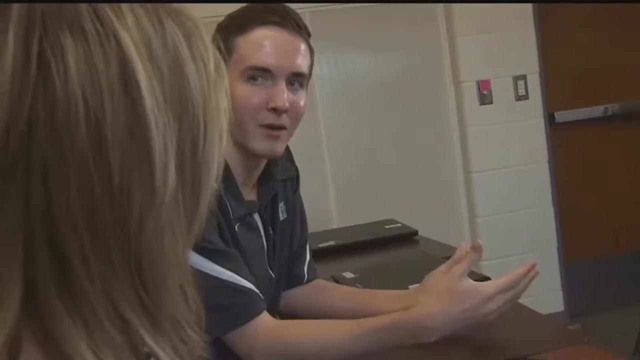 Wait, Oh no, So I forgot to add in the no key so that the guy stops eventually. We're lucky right now where you have the computer and you can run it back and forth, but back a long time ago you had to program for an entire week. 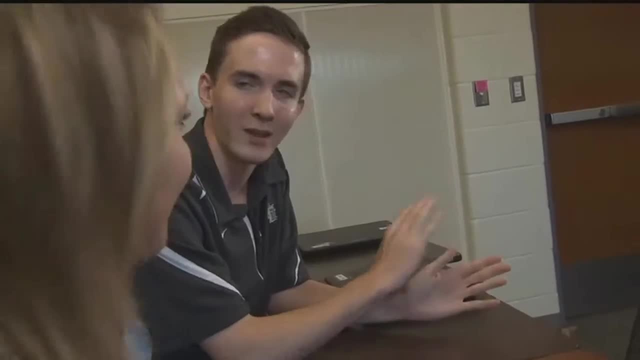 You get to test out your program once a week and you'd have to go back and you wouldn't get to test it out again for a whole other week. So it's very tedious work. In the future, do you think you want to do something like this when you get older? 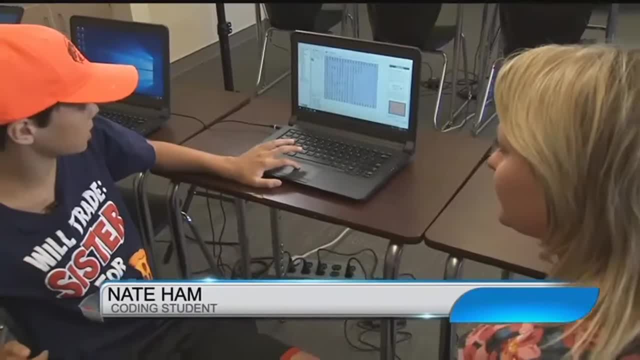 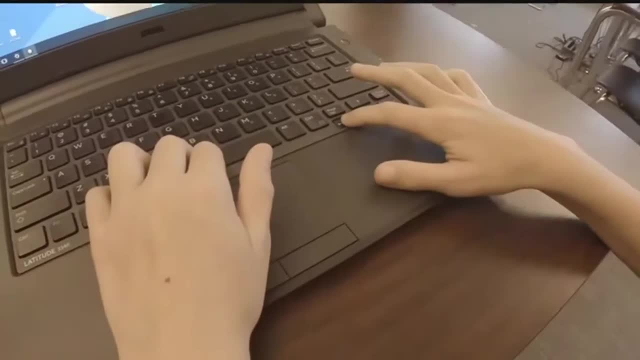 I don't know yet, but I'm just learning from this experience. Giving them this idea of method right now encourages them to go for it in the professional world And I think, almost confident enough that, no matter how confusing it may be in the start, 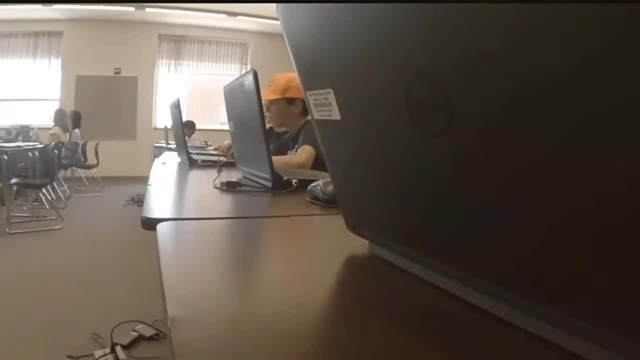 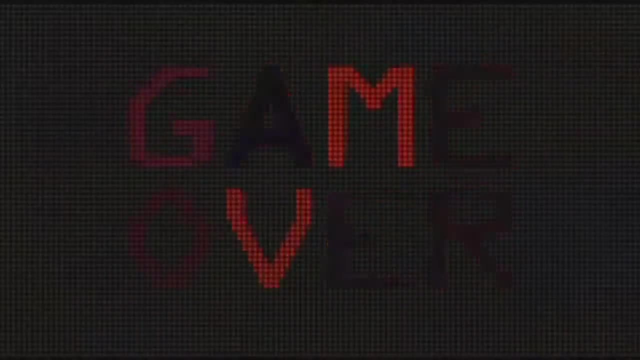 they see, even in just a week, how fast they catch on, that they'll catch on again too. I'm stuck. It looks like our character's a little bit too big to go through the walls there. Okay, coding is harder than it looks. 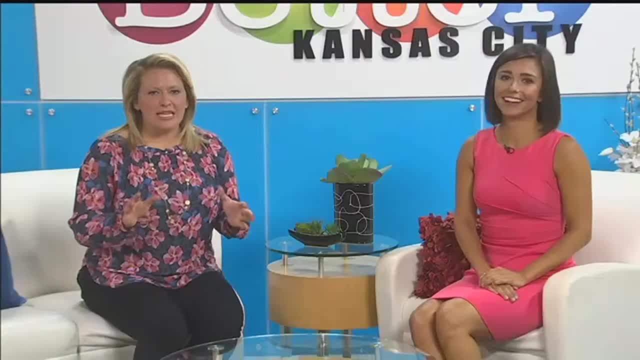 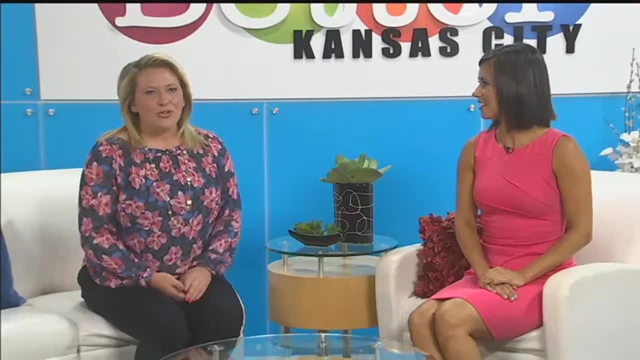 That's why it's good they're starting them young. These kids had the most amazing games like so intricate, And I'm thinking: how do you know how to do that? That's so impressive, But they do. Basically. I said: how early is it to start coding?